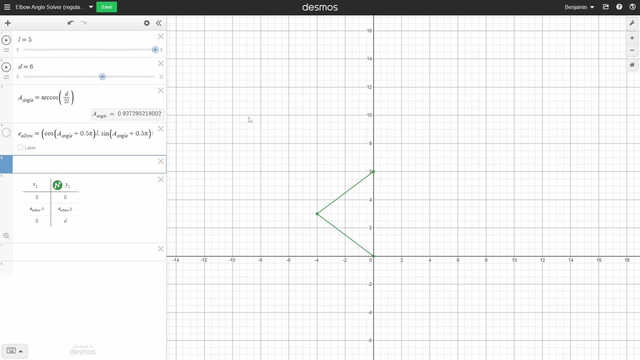 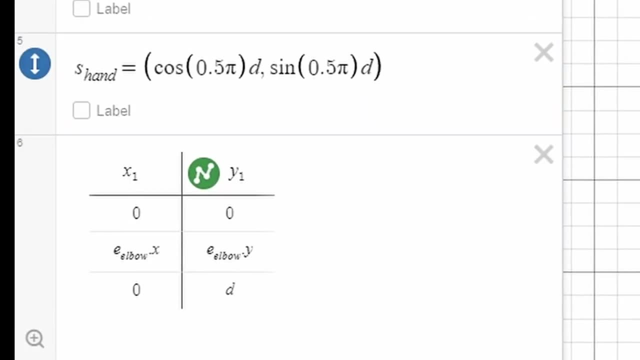 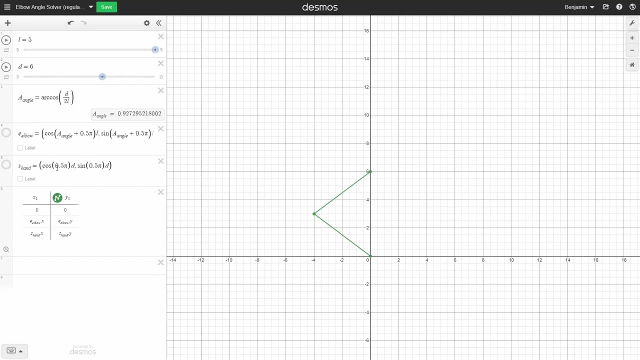 I'll set up a new vector and do the math for the angle of the end effector. I'll set up a new vector and do the math for the end effector position, so the hand position, As you can see here this time when we're converting the polar coordinates over to. 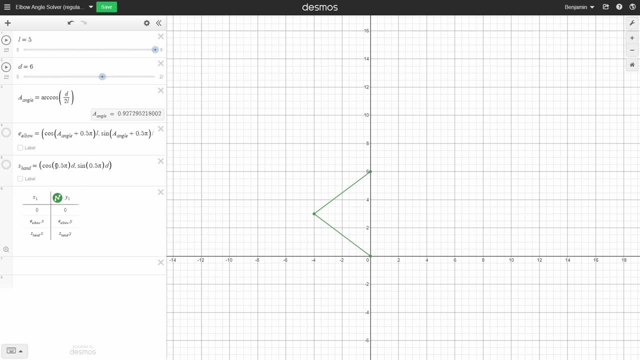 that get the hand's Cartesian position. we use just the angle, not the elbow angle, which is what is described up here. We use just the angle of the arm And we multiply it by the distance, this time instead of the length. Another thing we do here is, before we calculate the elbow angle, 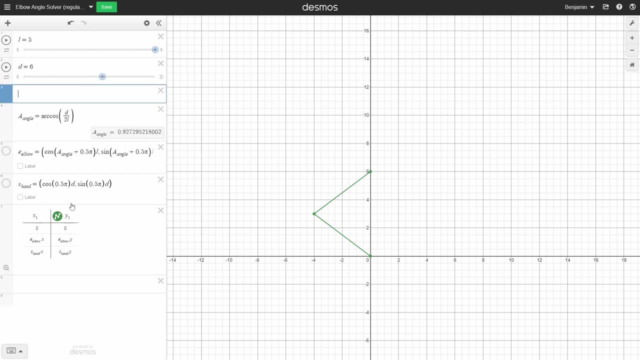 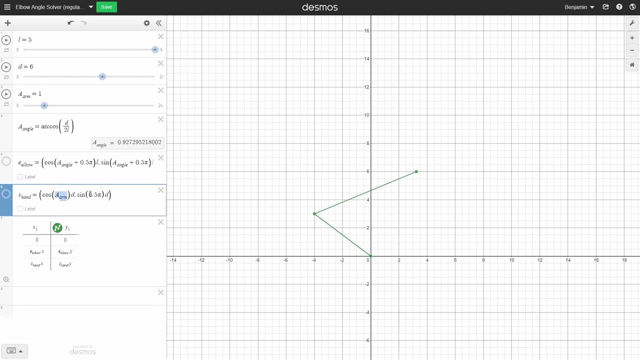 we can just get the angle for the arm. I'm going to constrain the angle in DiasMOS between 0 and 2 pi. I'm going to constrain the angle in DiasMOS between 0 and 2 pi. Now you can see here, nothing changes. 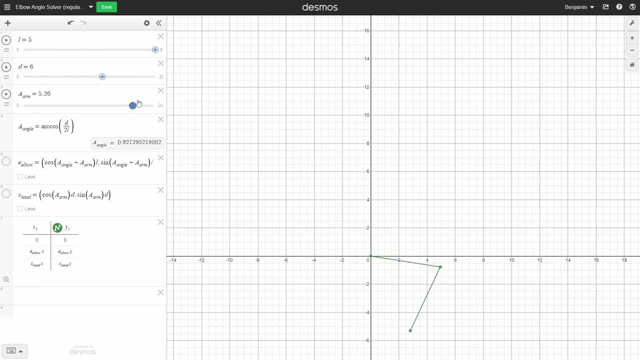 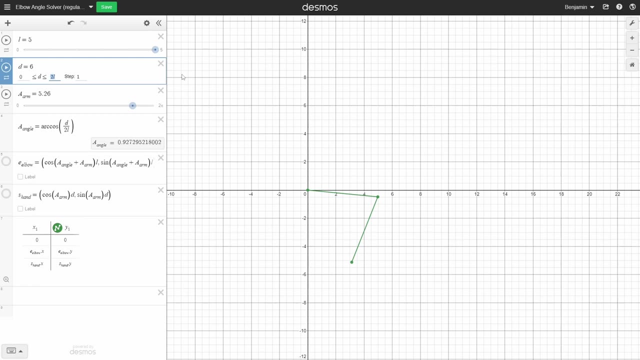 It's hard coded, but we are able to do the inverse kinematics at any angle. Here in DiasMOS the thing is, I'm able to constrain the distance, So here I made sure that the distance is never greater than twice the length of an individual. 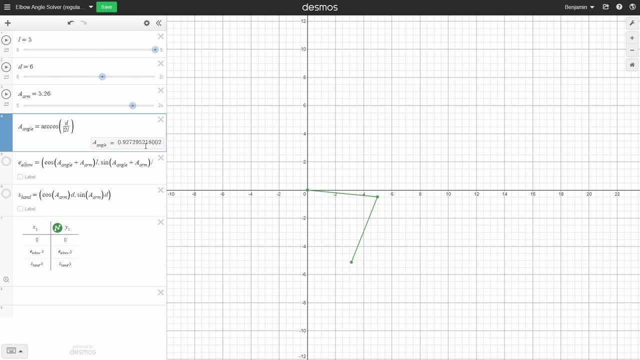 segment. So if you see when you're doing your Arccos calculation, you don't want to pass anything above 1 pi. You don't want to pass anything above 1 pi. You don't want to pass anything above 1 pi. 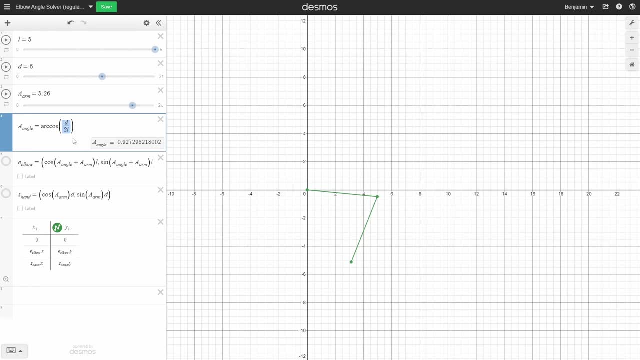 You don't want to pass anything below 1 pi, You don't want to pass anything. and if you see the angle, you get the interval below 1 pi or belowthe epsilon-1-1-1 here, or below, above 1 pi or below-1. and if you divide by zero, 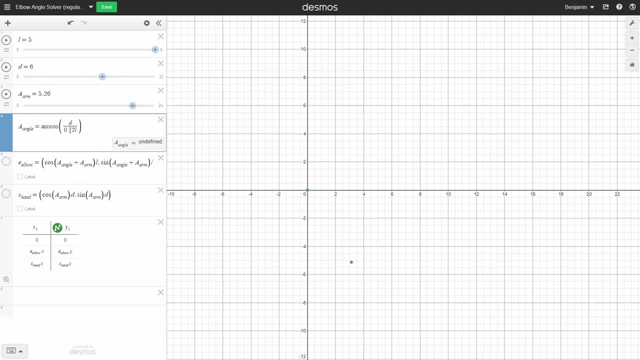 You're going to get an undefined error, or I guess in code you'd probably get a Like that. another thing is if the distance is too high, if it's greater than twice the length of an individual link, than you'll also get an error. 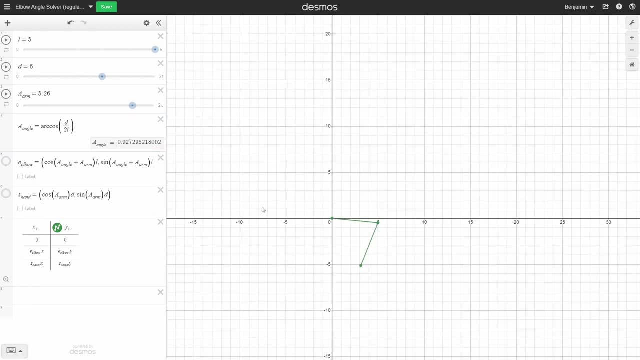 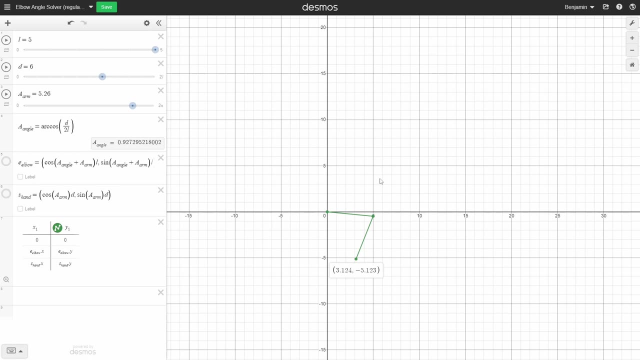 So here it's undefined. Here's the change in this: Harriet Brothers disappears. the same thing will probably happen in your code, so what you have to do is constrain the position of the end factor, and you should also just check to see if arc cost returns undefined. 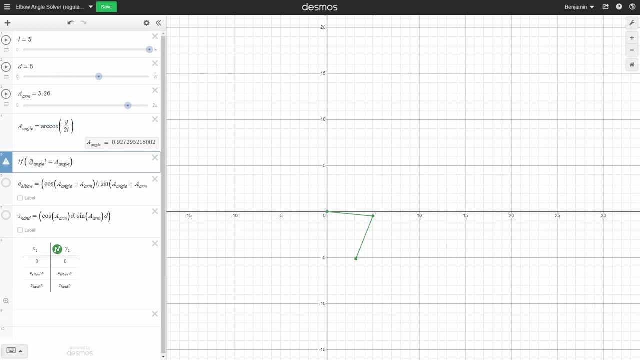 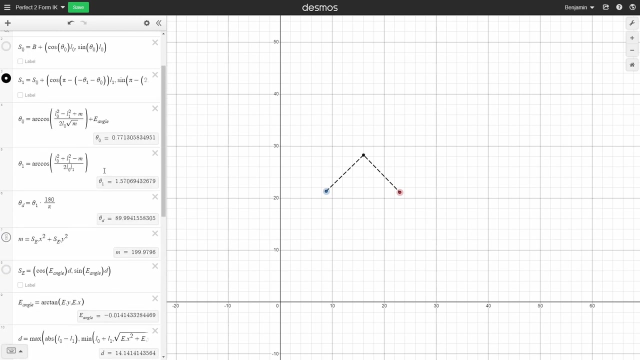 in code. you can just check to see if the angle equals itself, and if it doesn't equal itself, then you know it's not a number and you should just return zero in that case. so here's another example. i'm using what look like more complex equations here, but these are just the standard. 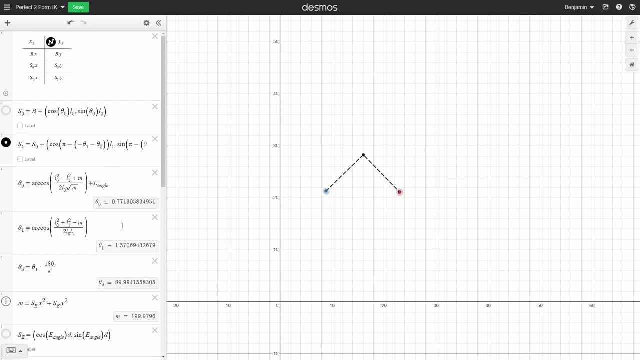 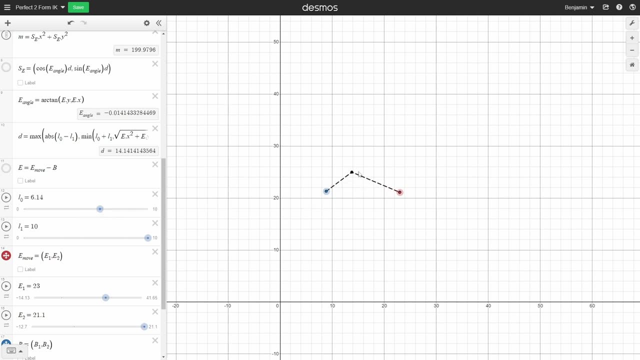 equations for analytical inverse kinematics, and also i have variable limb sizes here, so you can see that the limb lengths are asymmetric. the problem that's posed here is that the limb can't bend that far when the link lengths are asymmetrical like this, so you have to constrain- constrain the minimum distance and the maximum distance, and another: 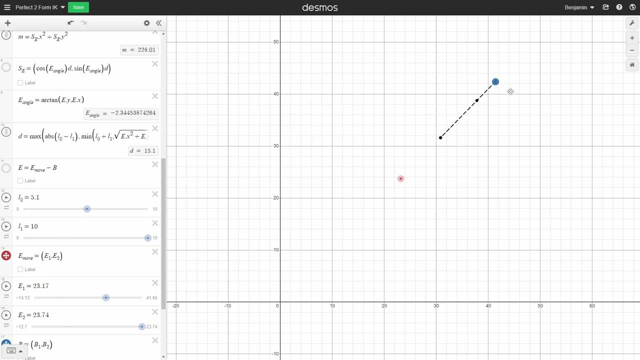 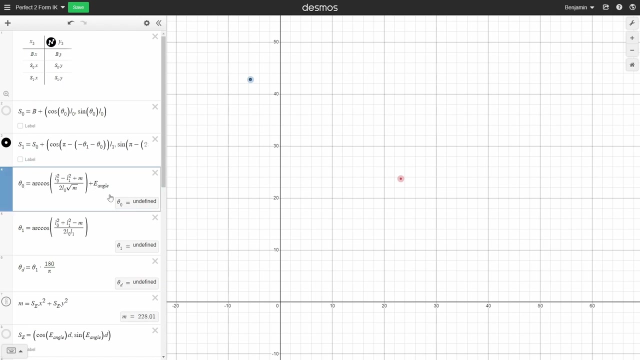 thing is i get these little flickers and i think this happens because of floating point precision. so at some point you're just gonna pass in your numbers into an arc cost somewhere and it's gonna return zero. so you can see here: everything disappeared. if you verify in code that it's. 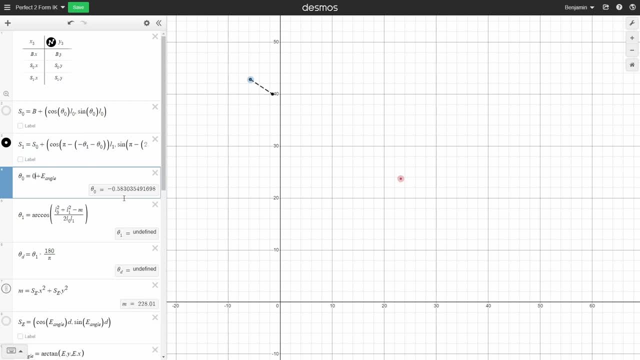 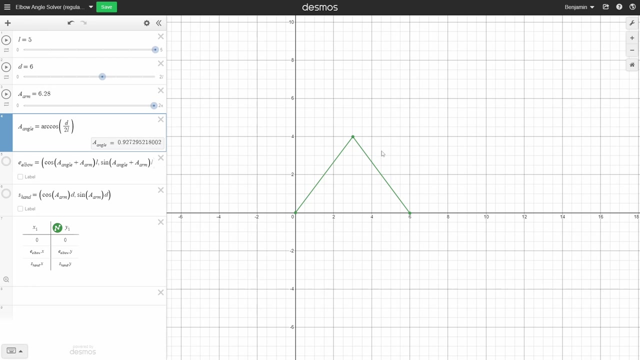 not a number, you just want to return zero. so if i just delete that, you can see the first link is pointing in the right direction and this only really happens when the angle of the elbow vector should be zero. anyways, i would recommend if you're getting into ik, to start with you should use a regular link. 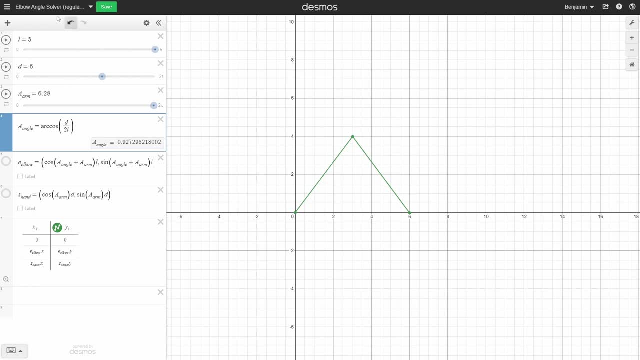 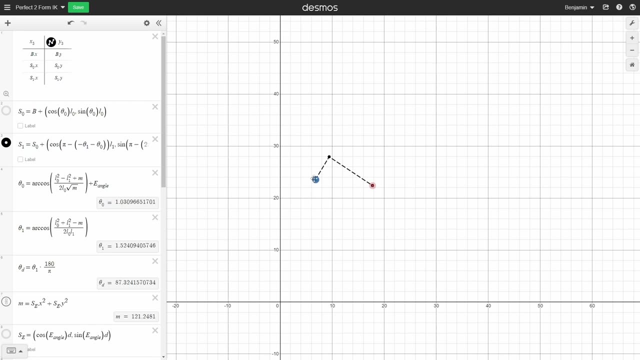 setup and just do it analytically, the way i've shown you here, and this way you'll at least understand the math. if you've taken a trigonometry class, unlike me, then you could probably use these functions, but, um, i would recommend that once you write them, you make sure to reuse them and just 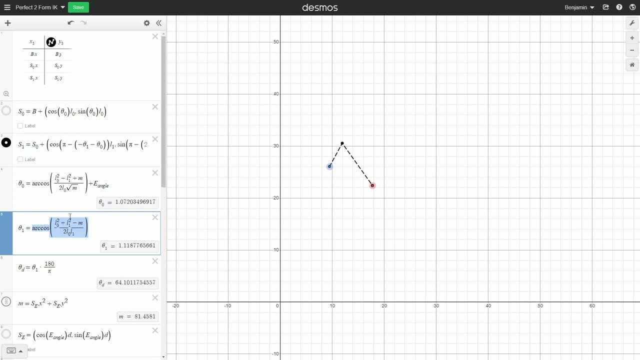 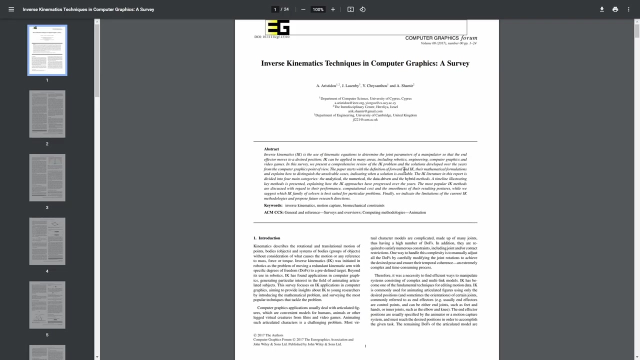 be careful while you're using them, or if you're advanced um, you could probably use the law of cosines. go through the steps in the law of cosines and try to work out this expression yourself, and then you can make up your own algebra in this paper, if you're interested in that.